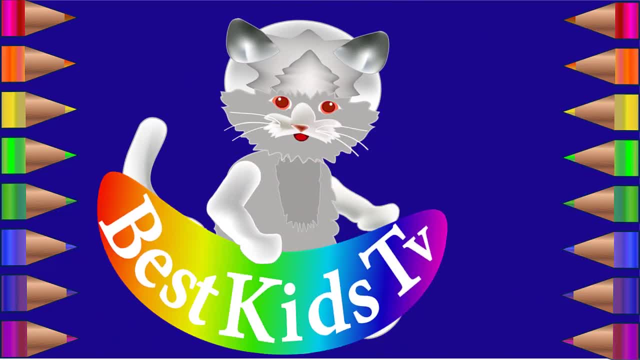 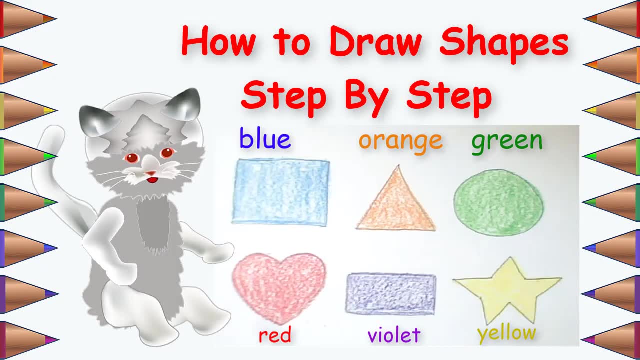 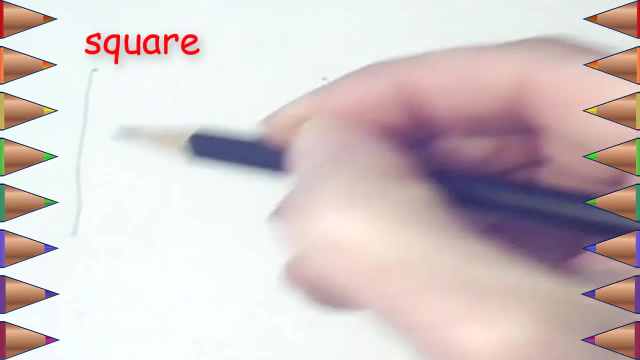 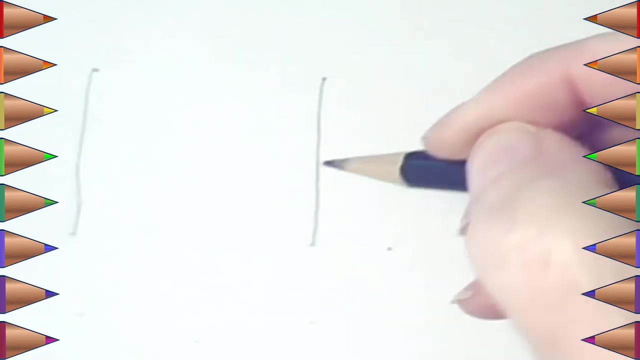 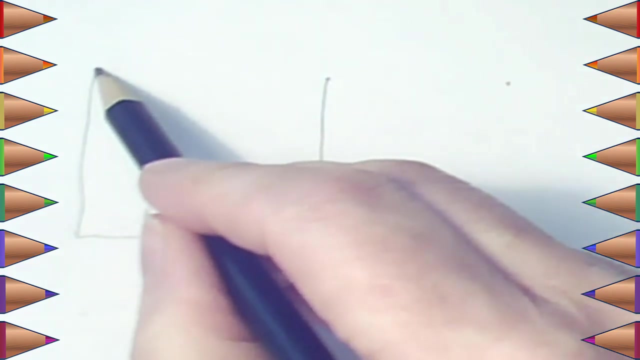 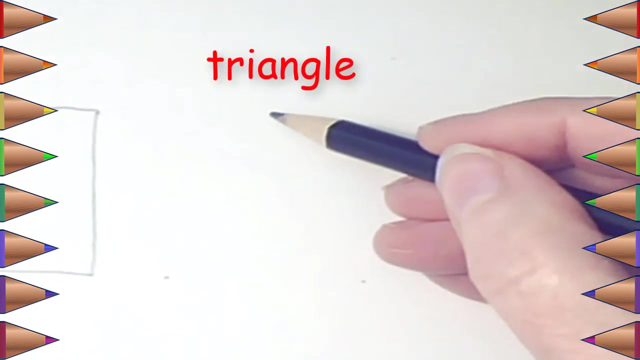 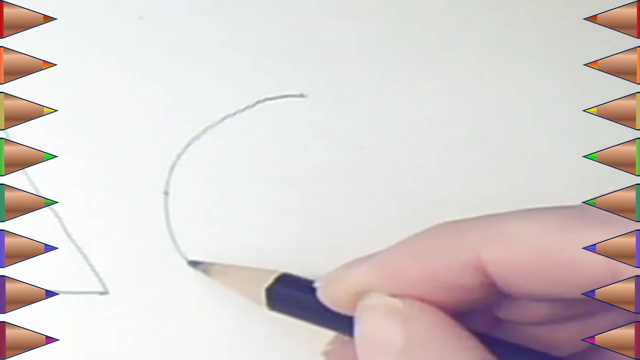 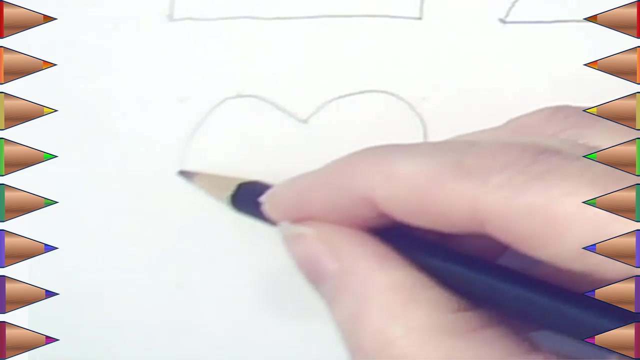 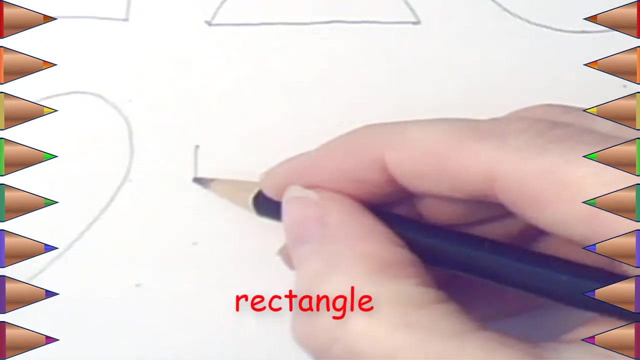 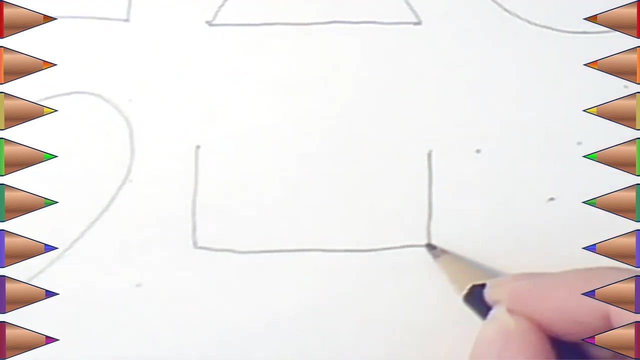 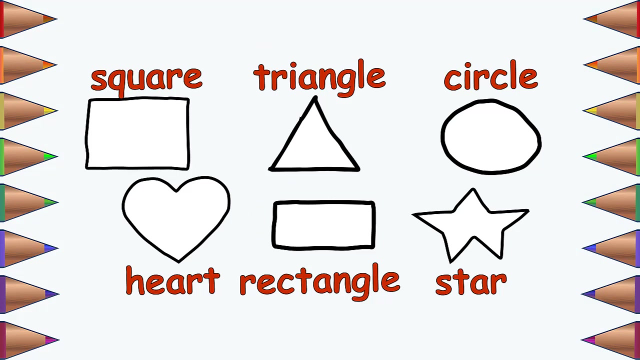 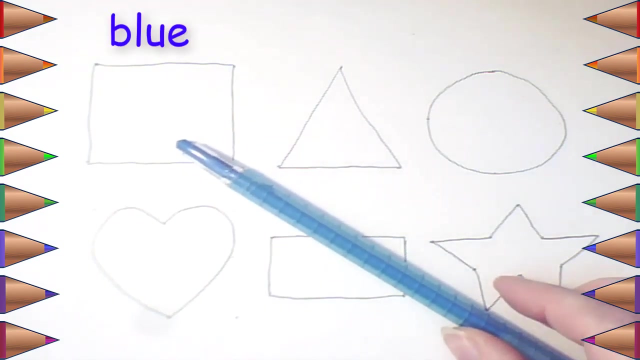 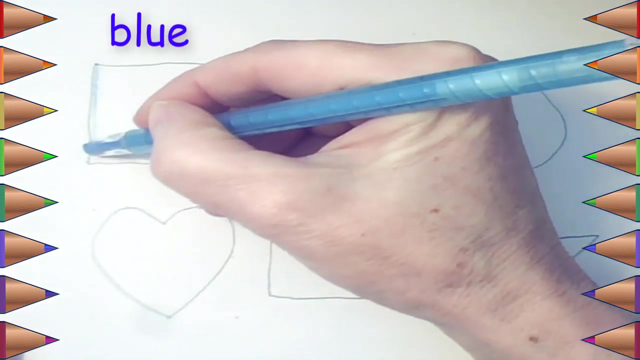 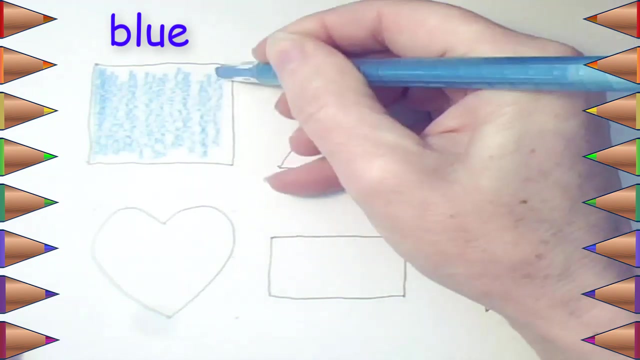 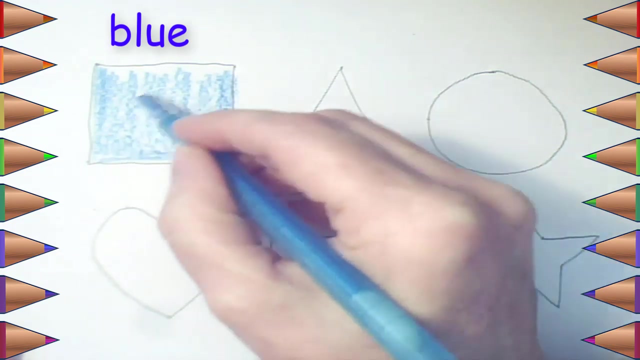 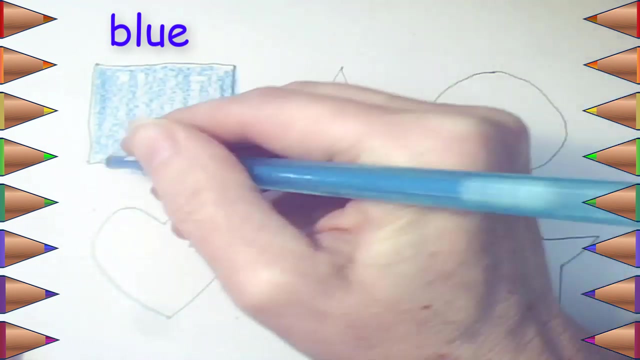 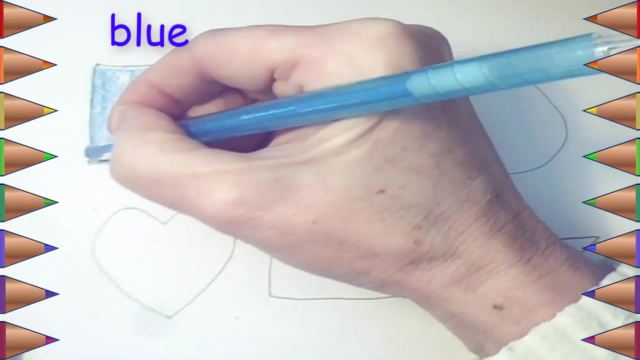 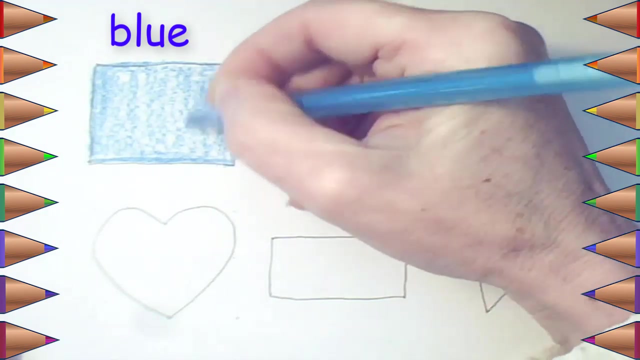 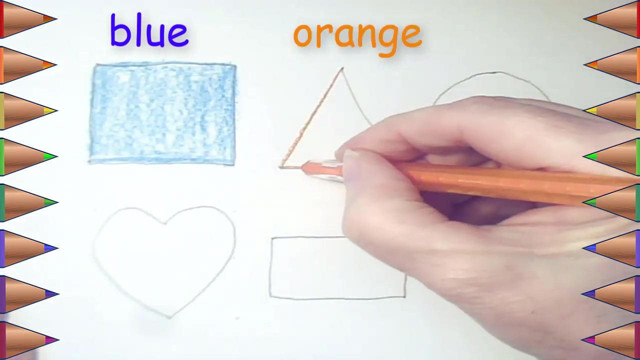 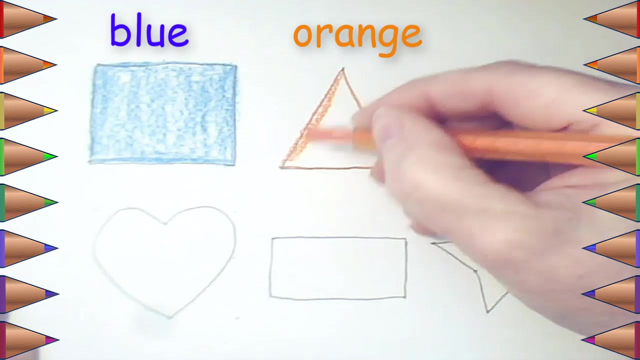 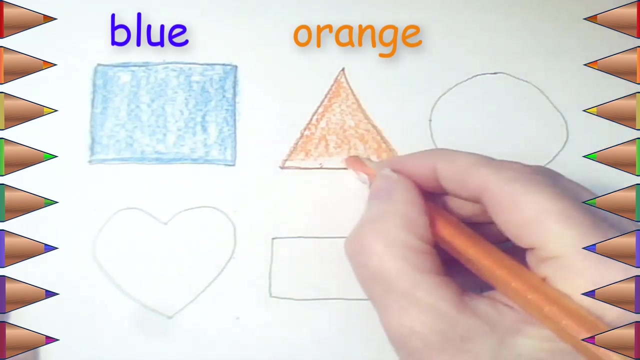 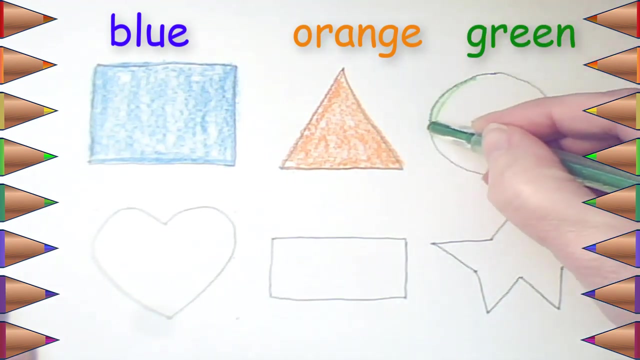 How to draw shapes step-by-step: Square, Square, Triangle, Triangle, Circle, Circle, Heart, Heart, Rectangle, Rectangle, Rectangle, Rectangle, Rectangle, Star Star, Star, Star, star. square, triangle, circle, heart rectangle, star blue. square, orange, Blue square, orange, Orange, triangle, Green, Blue, Red, Yellow, Green, Blue, Green, Blue, Blue, Green, Blue, Blue. 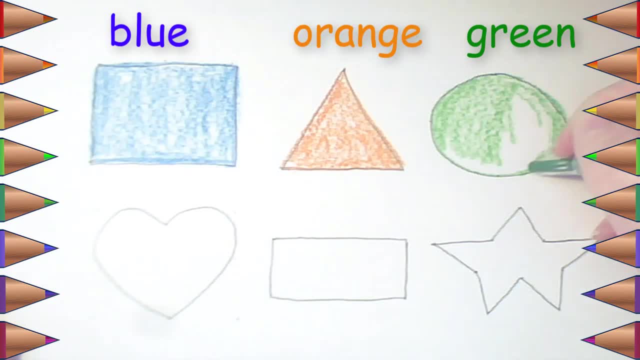 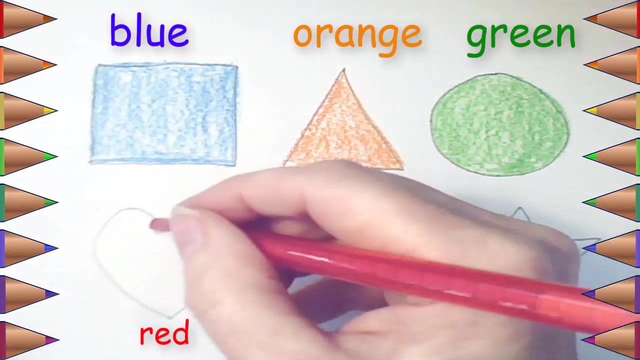 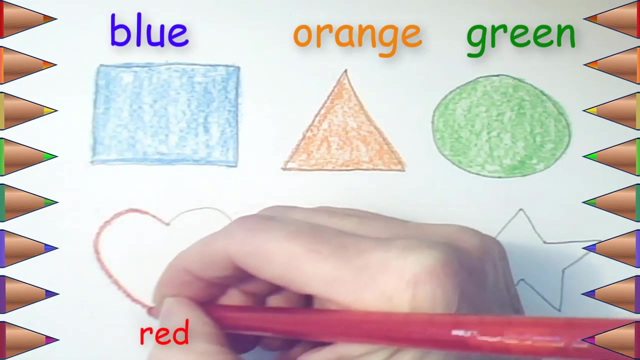 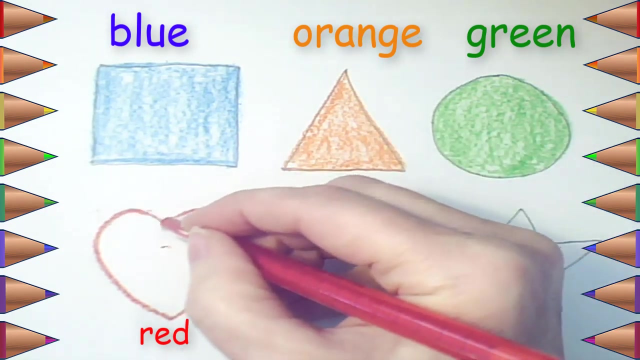 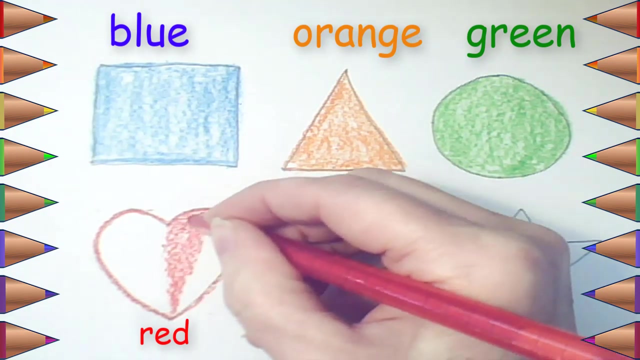 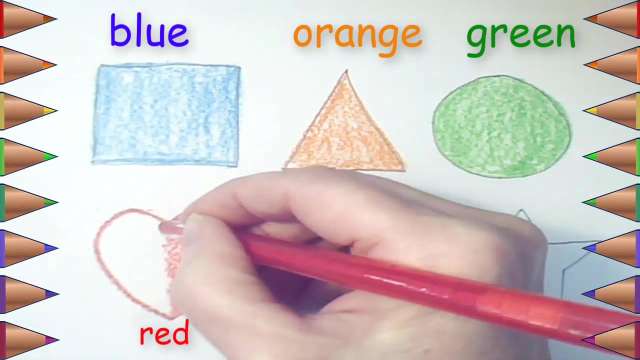 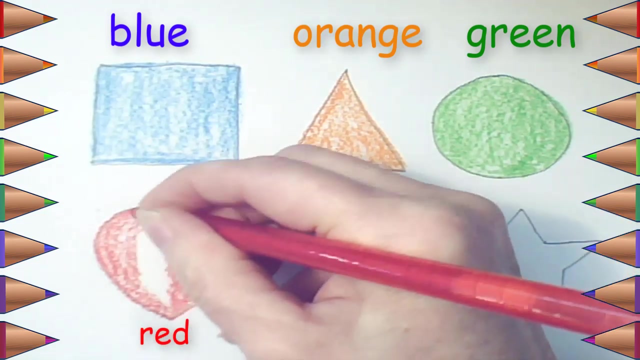 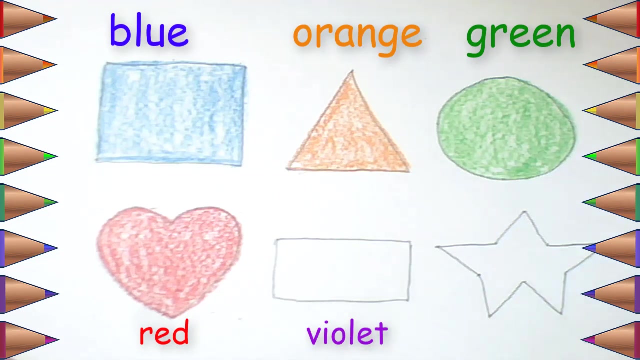 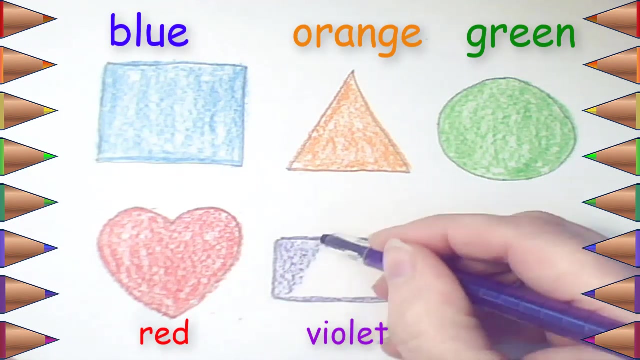 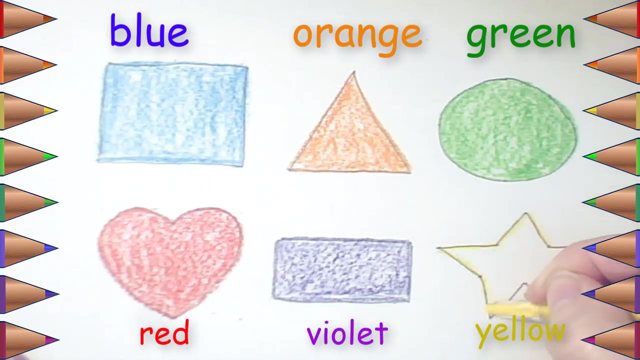 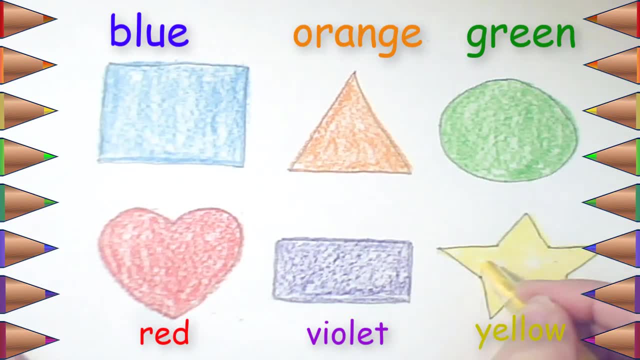 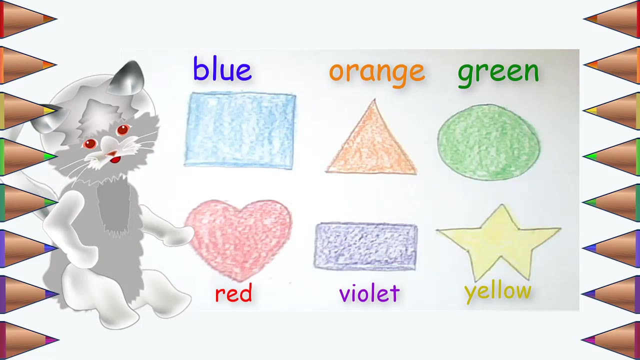 Violet, Violet Yellow Star. Thanks for watching, Bye bye. Thanks for watching, Bye bye.